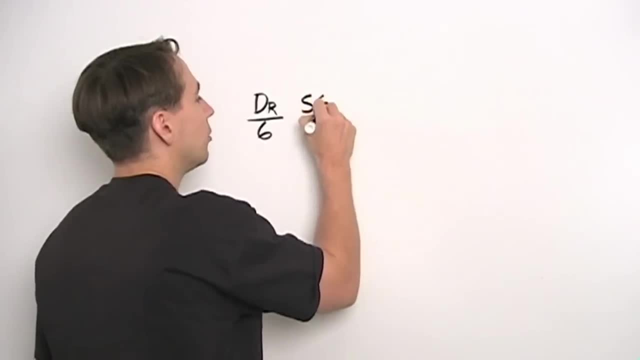 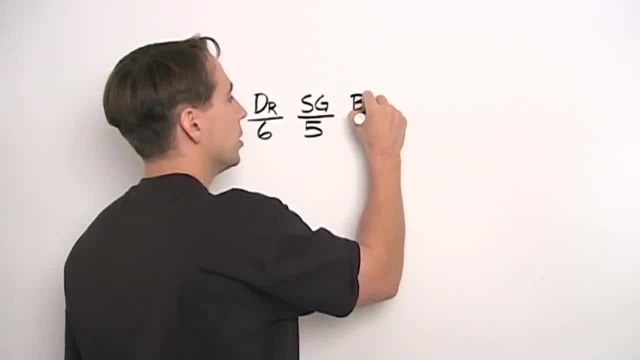 people left in the office. so we have five people to choose from for the shotgun seat, And then after that there are still four people to choose from to stick in the back seat with the pizza. So in total we'd have six times five times, four ways that we could. 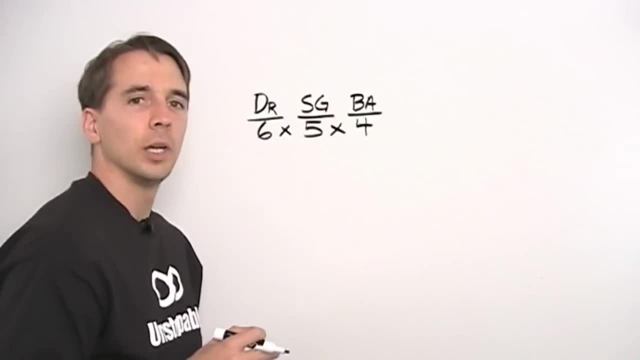 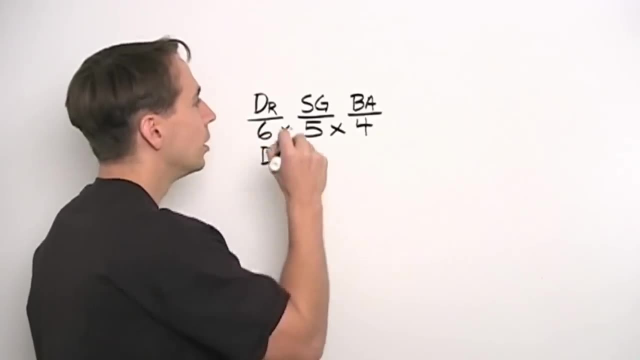 grab three of us, stick them in the car as the driver, shotgun and back seat and send them off to get the pizza. For example, we could have Dave drive put Larry in the shotgun seat and then put me in the back seat with the pizza. I like to be with the pizza. 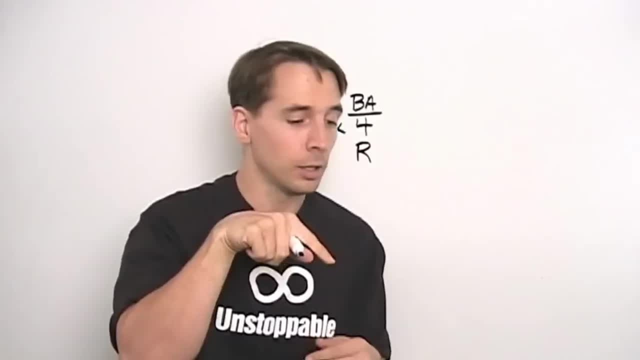 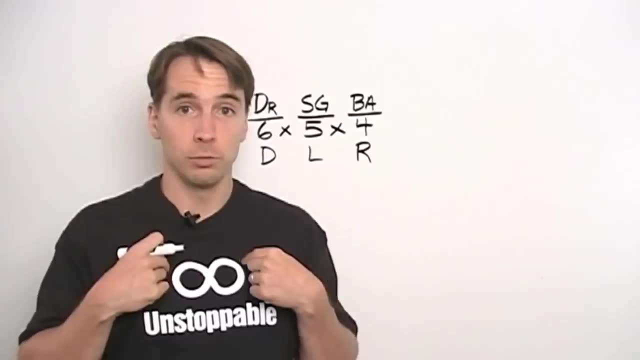 Now I should have introduced myself, but that's me. My name is Richard Russick. I think you can see it. Maybe it's there over there up there. I'm not sure where it is, I can't quite see. But, Richard, that's me R. So if we're going to drive, we have six times five. 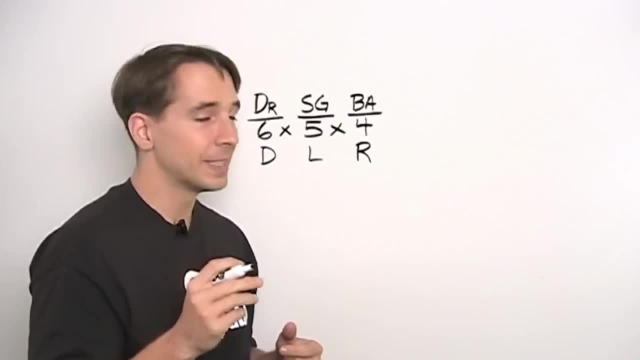 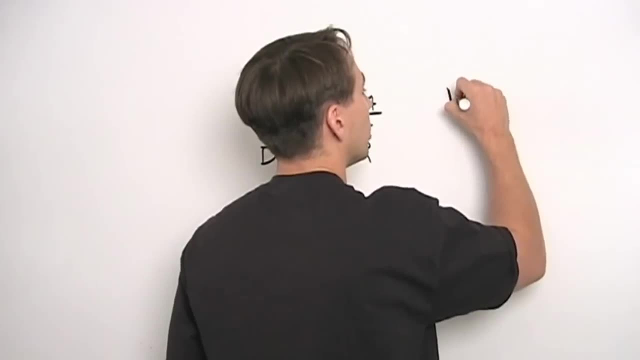 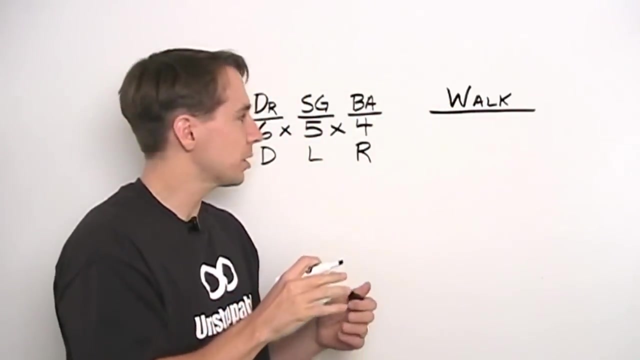 times four ways to go get the pizza. Unfortunately, as you know, gas has gotten really expensive so we don't drive anymore. Pizza place is close enough. We walk And we still send three people. So we have the six of us to go walk down. But the difference now is the order doesn't. 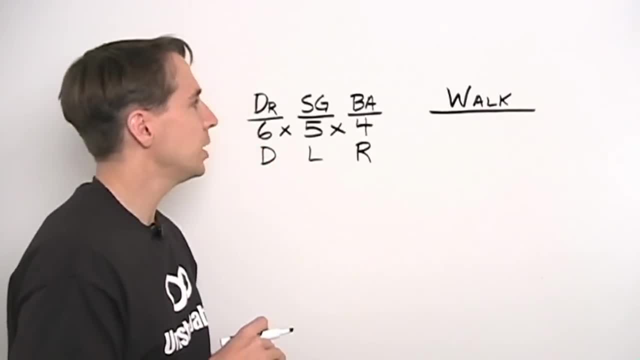 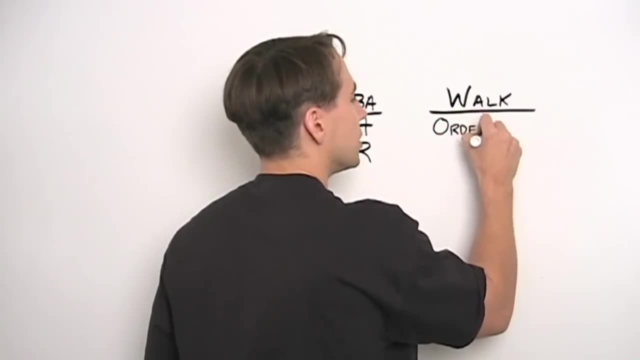 really matter. We don't have a driver of the group, We're just a group of three people going down to get the pizza. So the big difference here- and I'm going to write it down, that's how important it is- is the order doesn't matter. And to give you an example of how 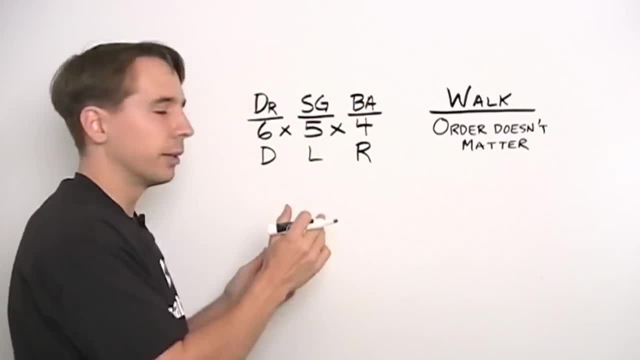 it matters over here. this isn't the only way Dave, Larry and I can get in a car. Well, Larry could be driving Dave in the shotgun seat and I'm still in the backseat eating the pizza you bought us. 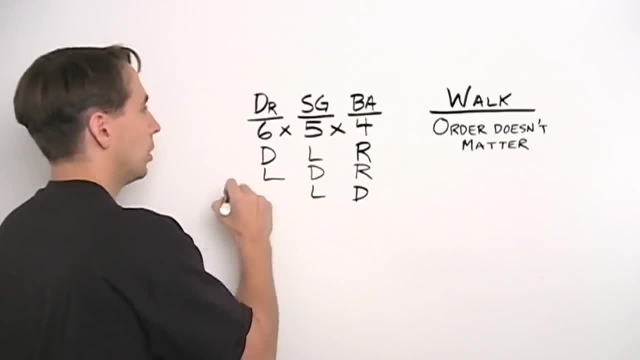 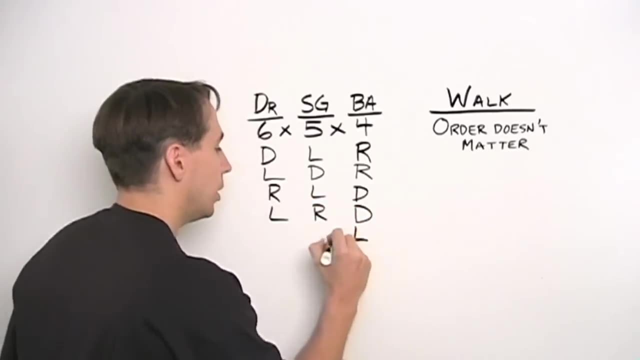 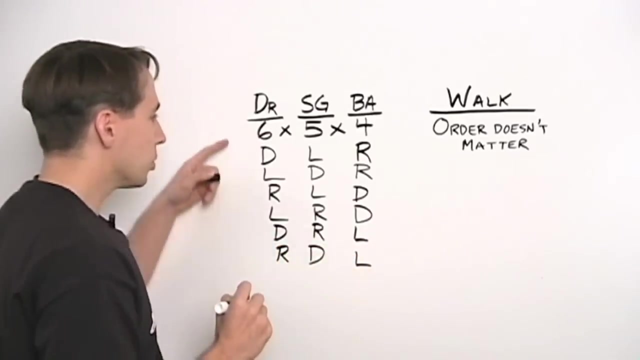 Or we could put Dave in the backseat and Larry in the shotgun and have me drive, Or Larry could be driving with me in the shotgun, Dave in the backseat, Or we could put Larry in the backseat with the pizza, And there are a couple ways we can do that. So we see here. 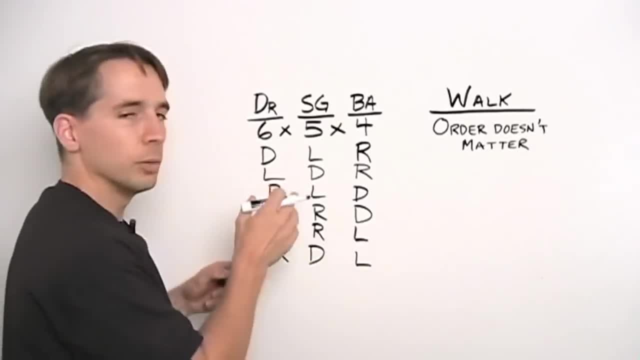 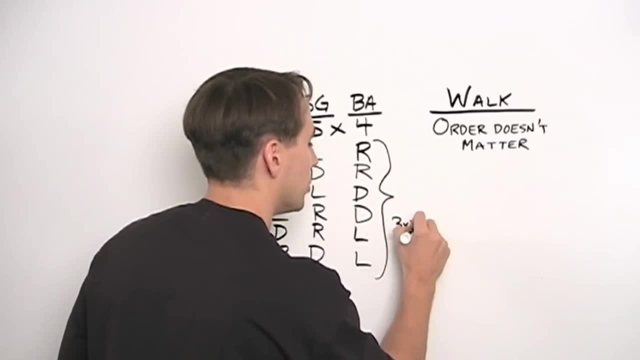 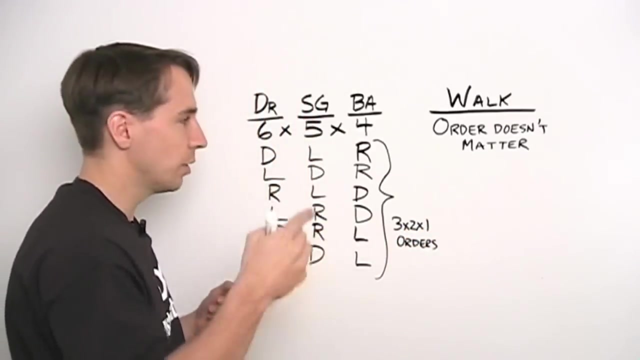 there are a bunch of different orders we can use to put Dave, Larry and me in the car. In fact, we see that there are three times, two times one orders, Because once you've picked three of us to put in the car, there are three ways to choose one of us to be the driver, and then there. 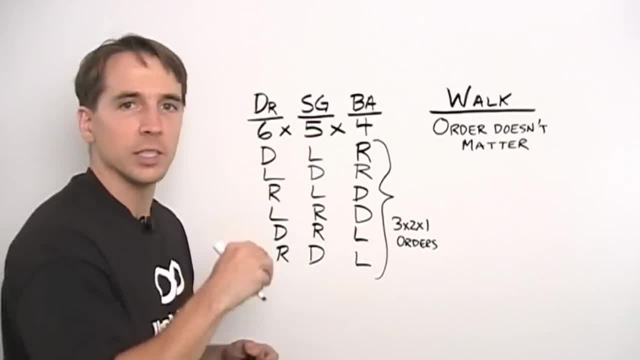 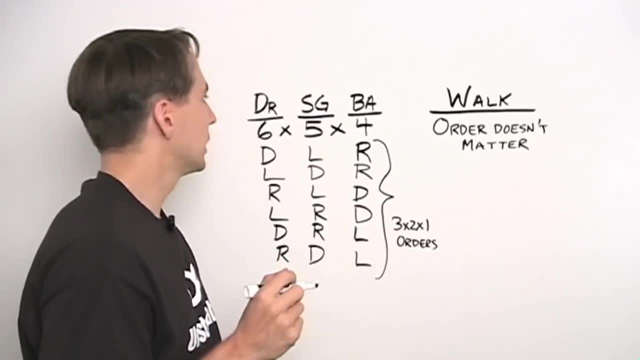 are two of us left to be in the shotgun seat and one in the backseat with the pizza, and I hope it's me, But over here when we're walking the order doesn't matter. So when we start counting the number of ways, we can pick three to send them to go get the pizza, well, we can start. 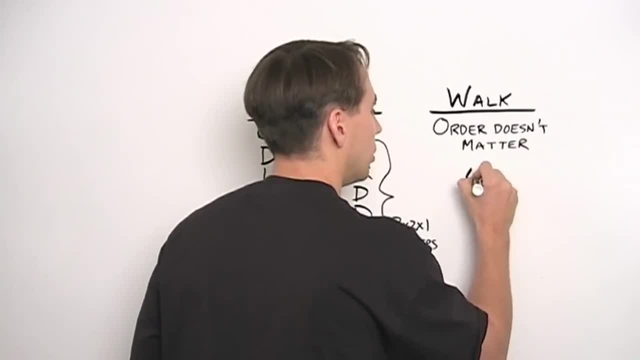 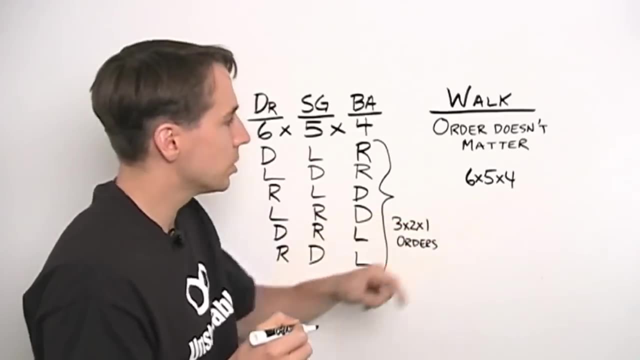 off the same way as before: Six times five times four And then choose the first person. There are six ways to choose the first person, five ways to choose the second, four ways to choose the last, But the problem here is we're over-counting. 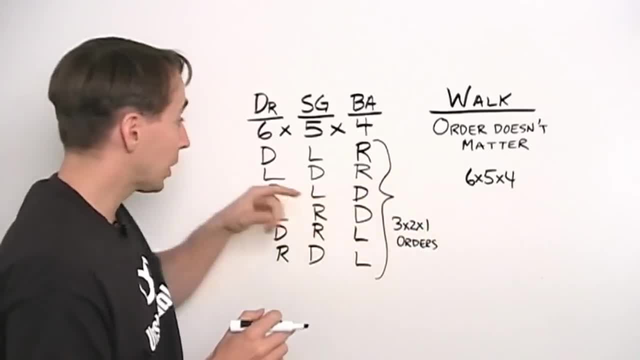 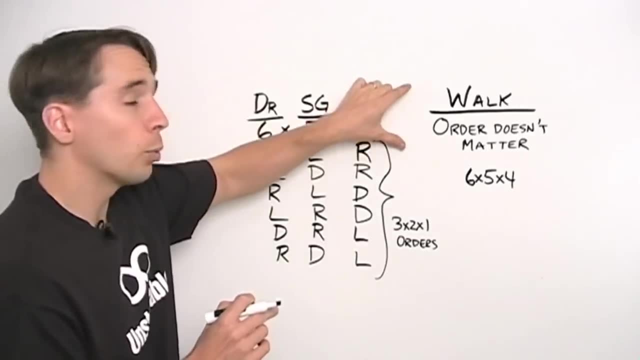 For example, Dave, Larry and I are counted. here. we're counted six times, And we see that over here We're counted three times, two times, one times, And those are all different when we're driving, but when we're walking they're all the same. So we only want to count. 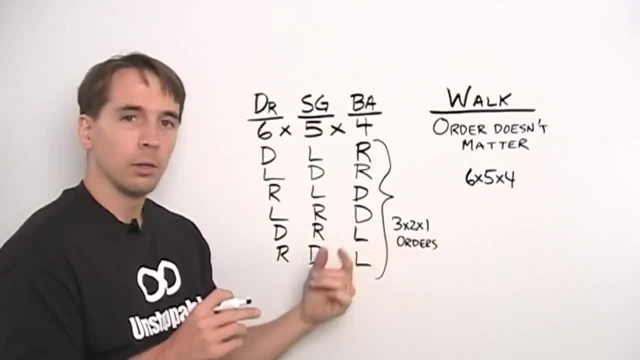 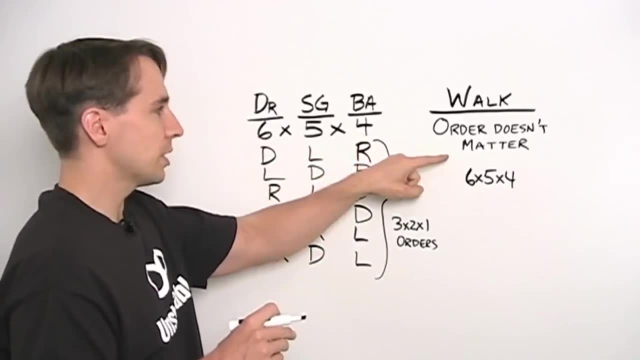 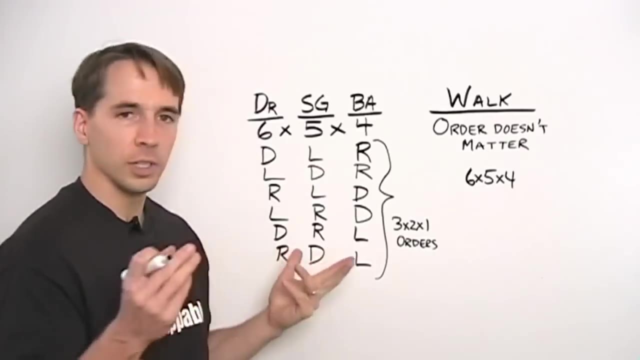 this once over here. but six times, five times four counts it Three times, two times, one times. That's a problem. In fact. every single group, every single group of three people gets counted three times, two times, one times. when we do six times, five times four, We only want to count it once. We count everything six times. 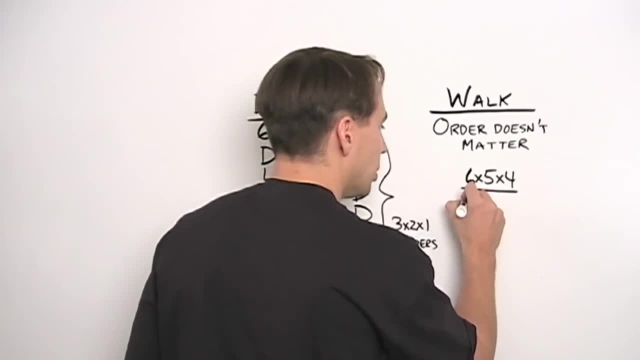 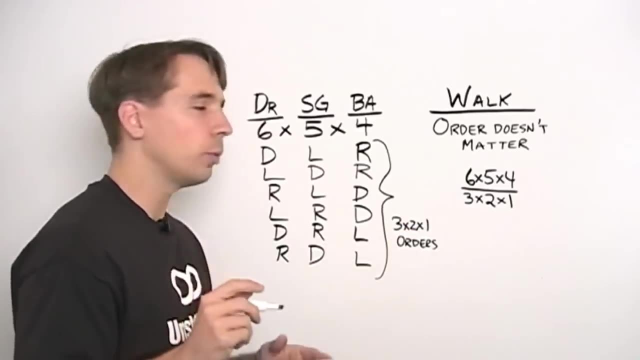 We know how to fix that. If we've counted everything three times, two times, one times, all we have to do is divide And then we'll count everything exactly once and only once. And that's the whole goal. Again, the whole difference between these two. 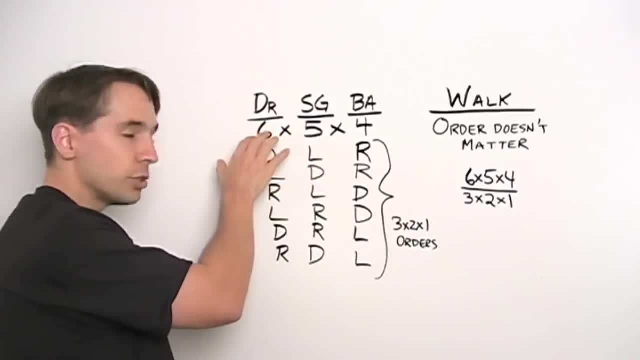 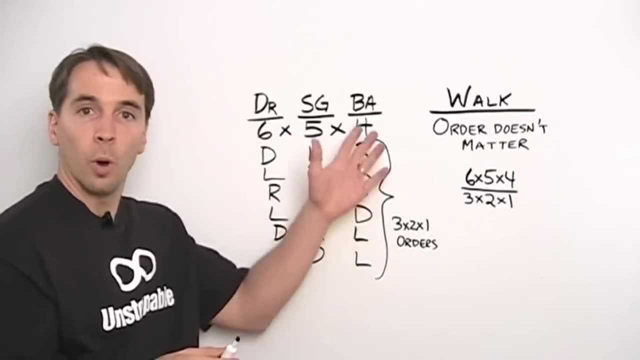 So when we're getting in the car, order matters: First person's the driver, next person's shotgun, next person's backseat. So these are all different when we're getting in the car, But when we're walking they're all the same. The order doesn't matter. 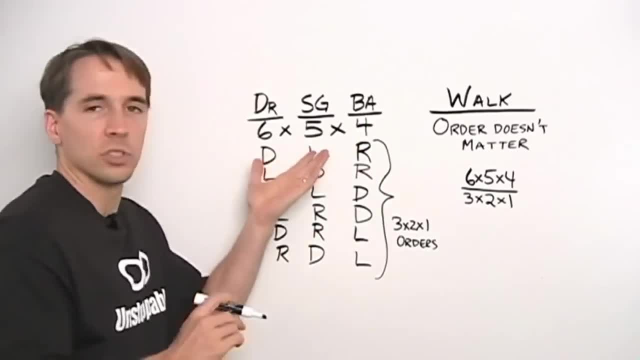 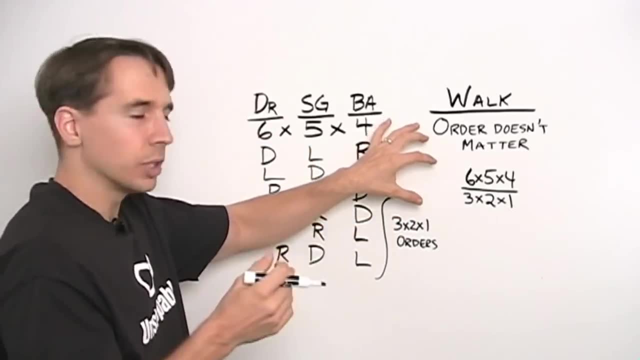 Now, we've seen this before. We gave it a fancy name- permutation- when really it's just multiplication. We've seen this before, but this is something new, And in fact, this comes up where you're choosing from a group and order doesn't matter. This comes up so much that it has a special 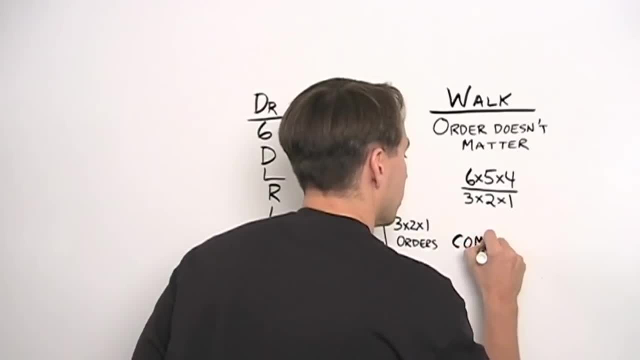 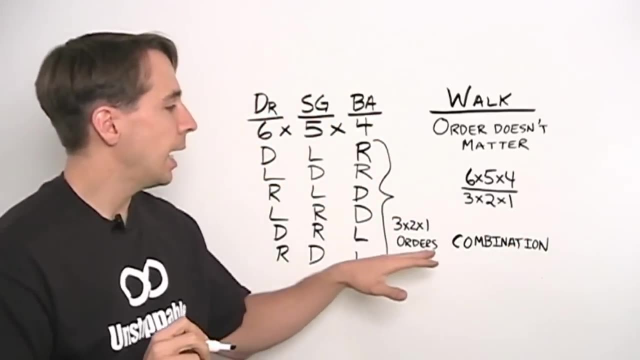 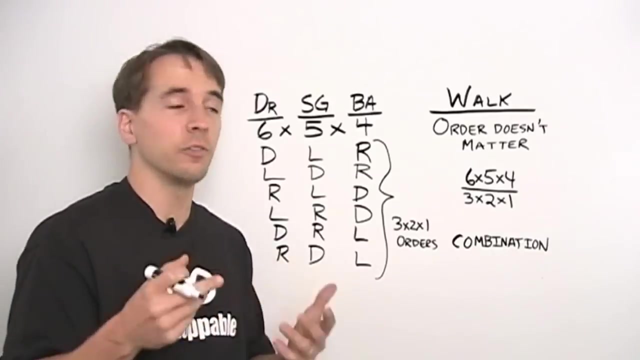 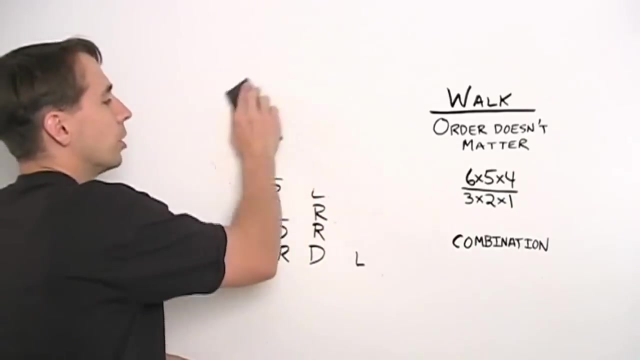 name, I'm going to write it down here: Combination, And we're going to talk a lot more about combinations, because you use these so much in counting. they become just another operation, like multiplication or division, addition or subtraction. They become so common that we even have some special notation for it.